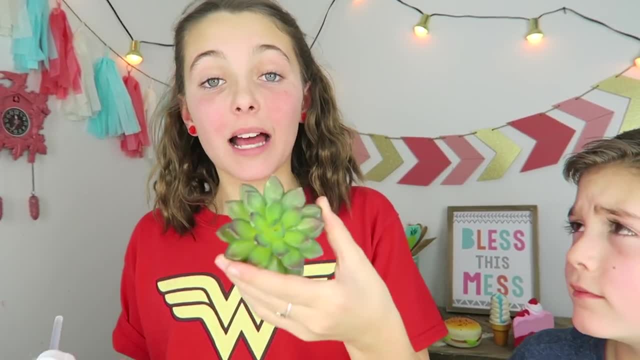 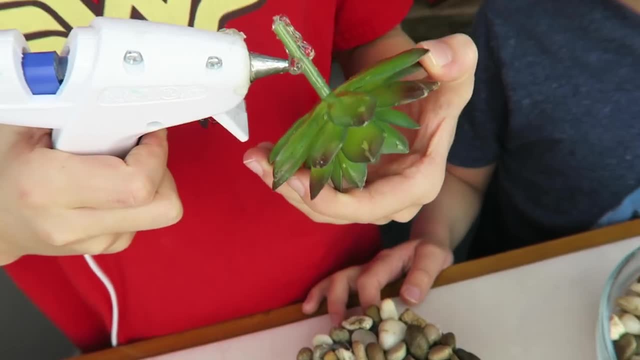 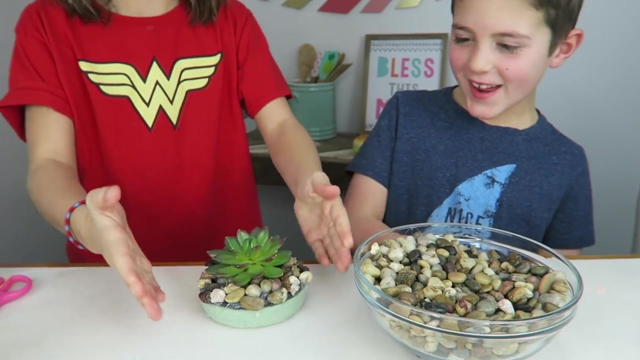 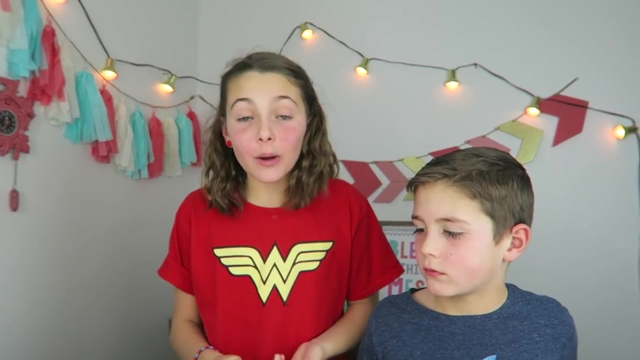 plastic flower and putting hot glue all over the stem, Then boop right in it goes, Push it in. It kind of looks real. Yeah, it looks pretty cool. Yeah, it looks pretty real. Okay. so now what we're going to do is get. 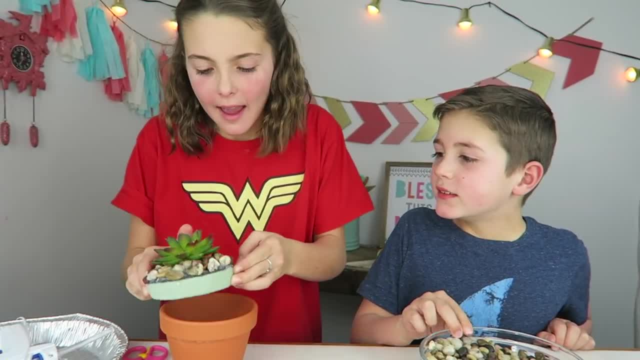 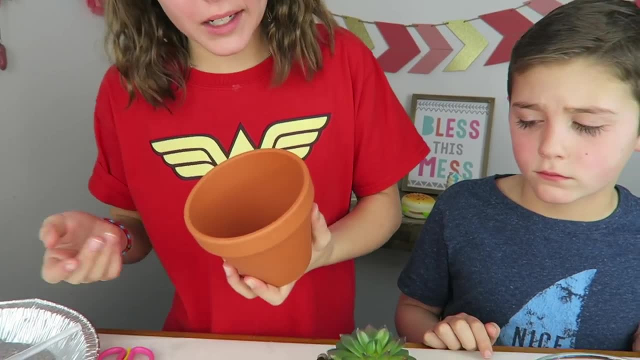 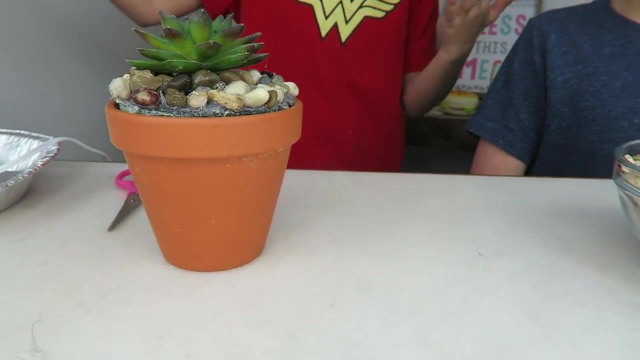 our flower box and place it in there. When we place it in the pot, there's going to be this little space at the bottom. That's where you're going to store all your stuff, Your secret stuff. It actually looks like a plant and a bowl of rocks. 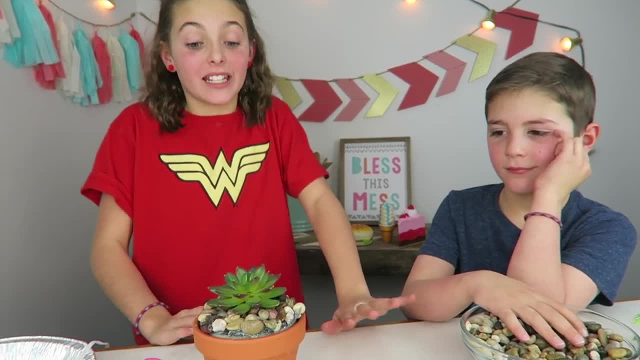 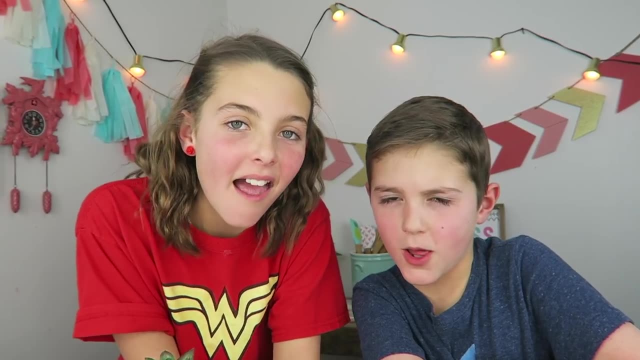 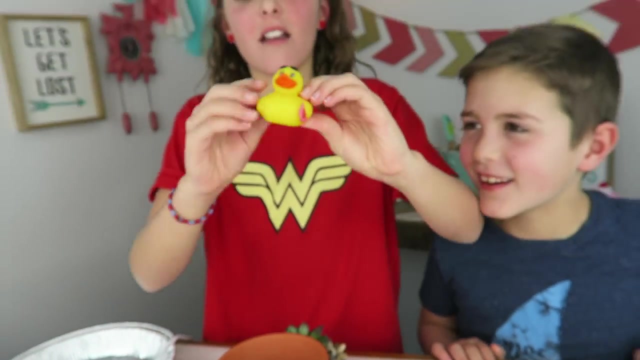 That is cool. Nobody will know that. it's totally hollow in the inside. What should we put in the secret stash plant? Comment down below. Let's see what's inside. This is fun- A rubber ducky. Okay, let's do. 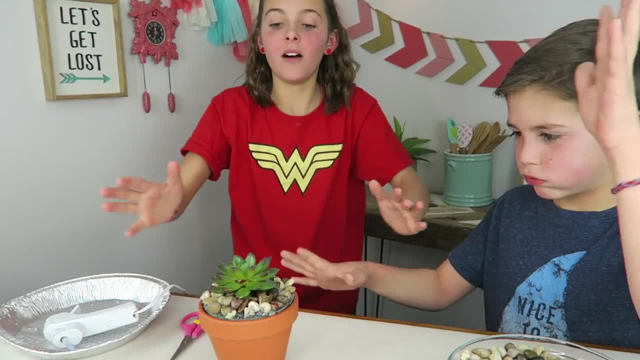 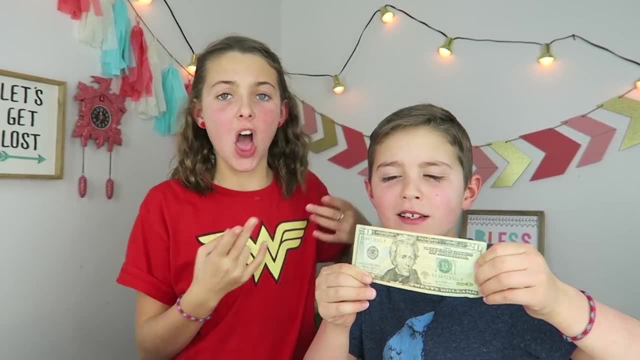 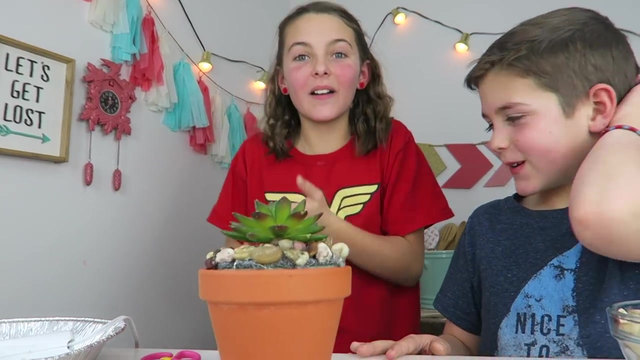 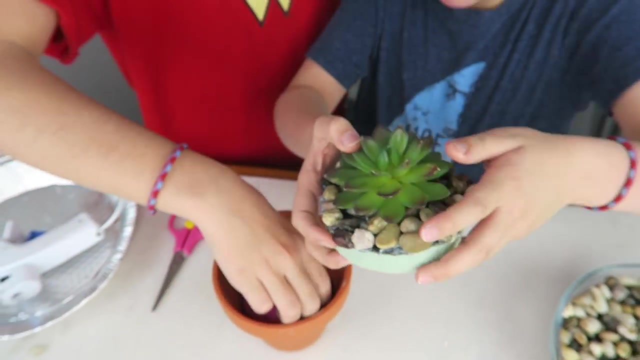 another one. Okay, let's see what we got. Let's see what we got. Dollar dollar bills, yo Oh, Bippity, boppity boo, You do it this time. Let's see what's inside A bubble gum. 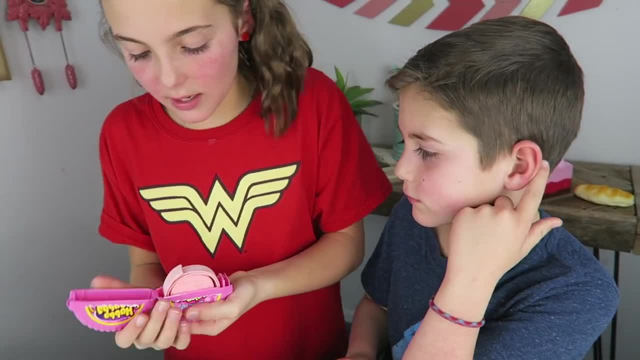 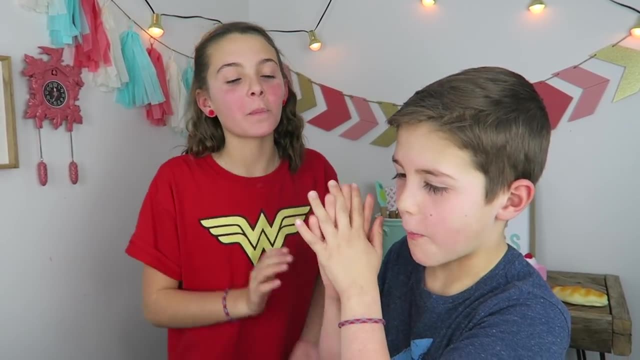 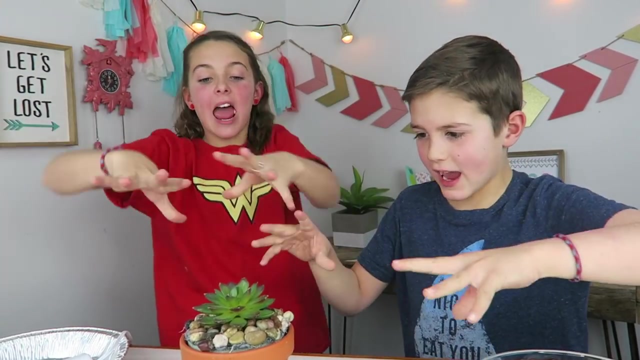 Tape roll, Woo, Let's have a piece. Oh yeah, Snap, I love this stuff. Okay, put the lid back on magician. Let's see what's inside. Alakazam, A band-aid. Oh, Axel, do you have a boo-boo? 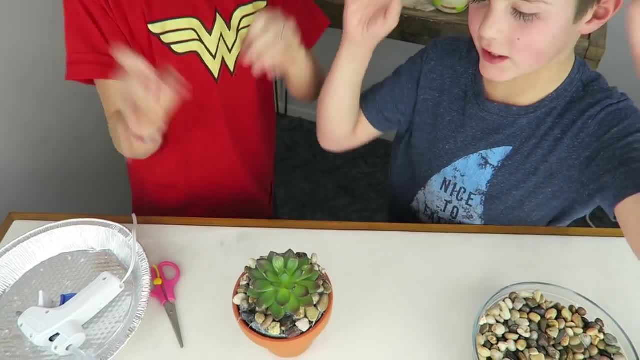 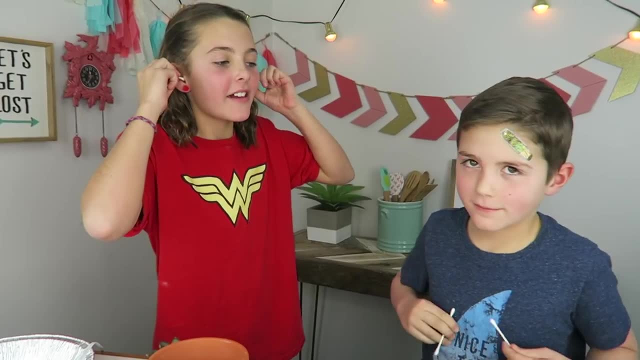 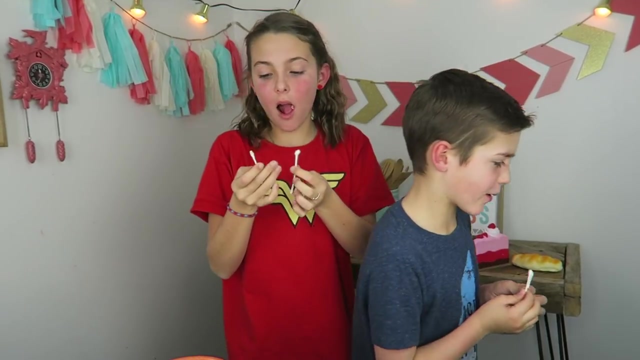 Okay, let's see what we have now. Alakazam Q-tips. Axel, do you need to clean your ears? I am Frankenstein. This feels good Garbage. It's over here. Okay, Bippity, boppity.